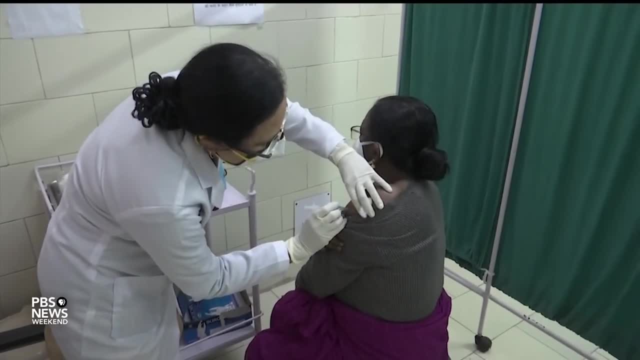 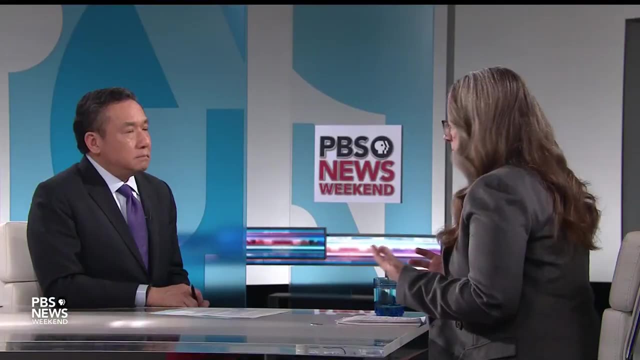 And that's what we're seeing right now. The pandemic and misinformation have combined to sort of really see this decline in vaccines for both of these infectious diseases. Thinking about just sort of the chaos that the pandemic gave us, a lot of people weren't getting. 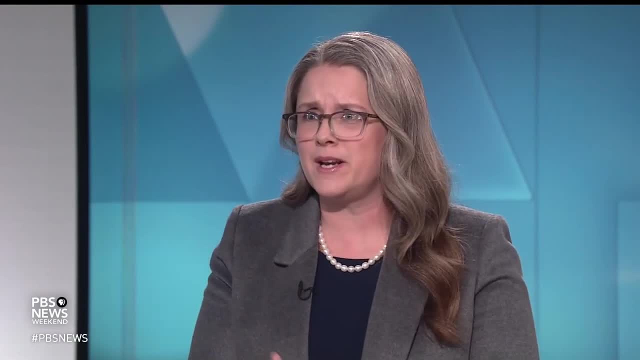 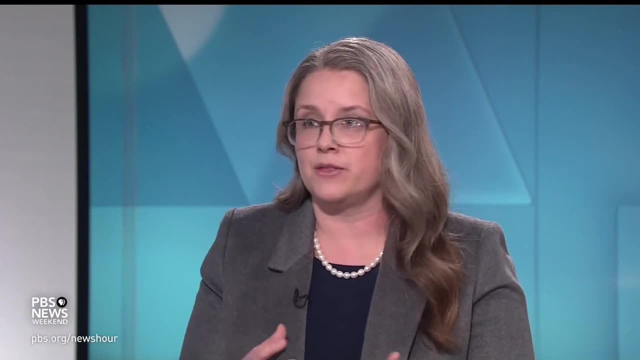 scheduled childhood vaccines for their kids. People were afraid to sit in waiting rooms, exam rooms, And we saw that and we're still sort of working our way out of that And then thinking about the role that misinformation has played in sort of undermining people's confidence in that we're still dealing with that mess. 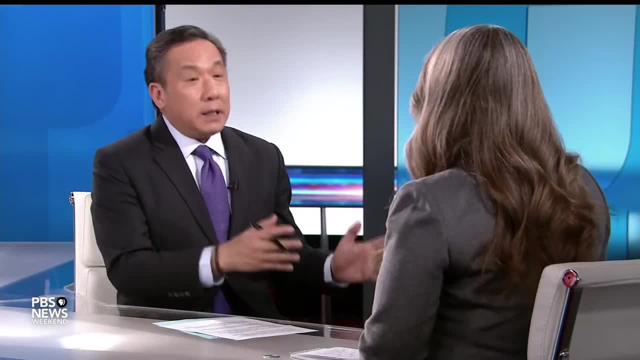 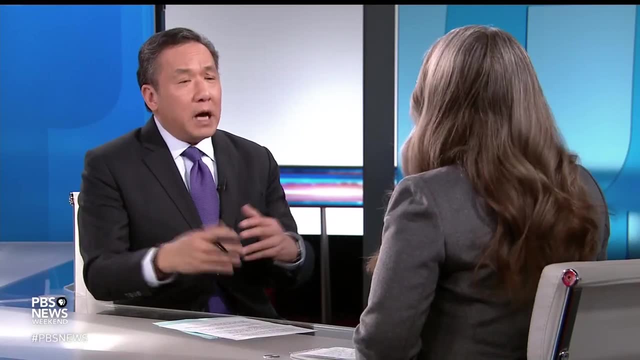 JOHN YANG. Some vaccines have been with us for generations, But looking back in history, looking at when they were first introduced into the public health system, they were the first to get vaccinated. JOHN YANG, Was there the same sort of misinformation then, or is that something a new phenomenon? 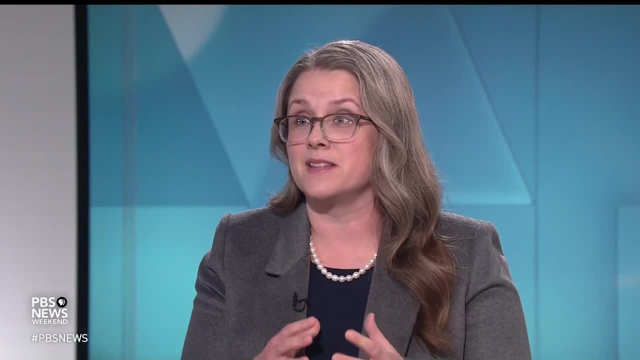 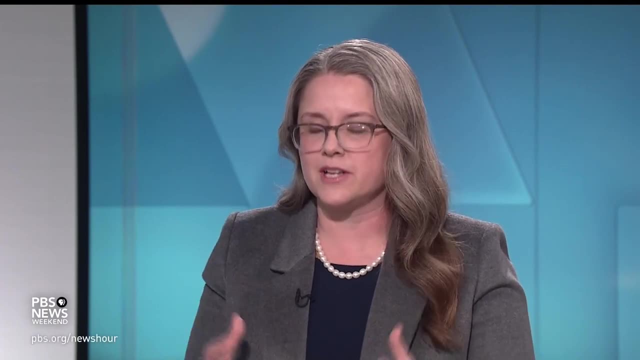 LAURA BARRON- It's kind of wild to think, You know, infectious diseases have been something that humanity has been dealing with since before we were able to record history right, And some of these diseases are, you know, we're just kind. 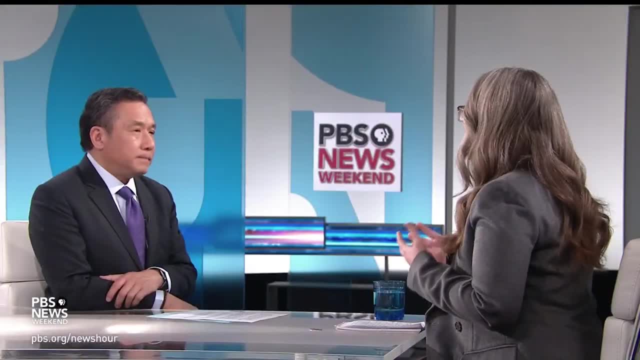 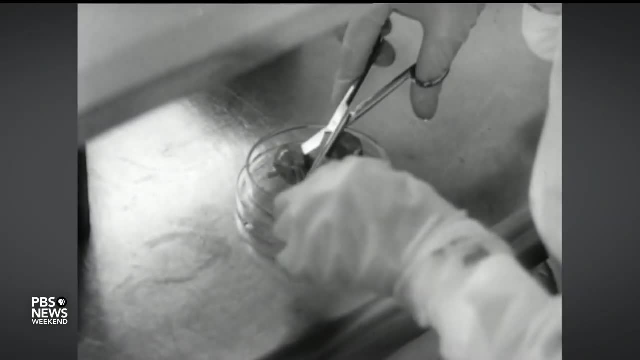 of starting to wrap our arms around. Take polio, for example. The ancient Egyptians were dealing with polio right, And it wasn't until the 1950s Dr Jonas Salk started to deploy a vaccine, starting in a school in Pittsburgh. 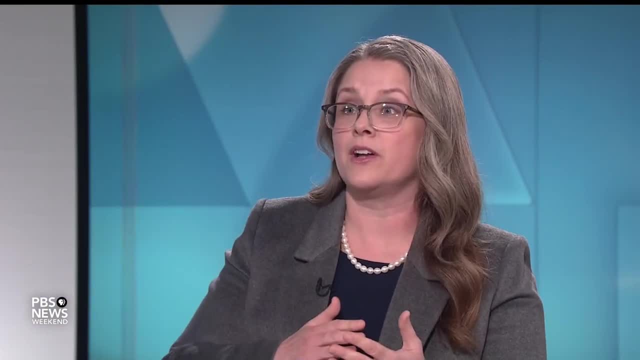 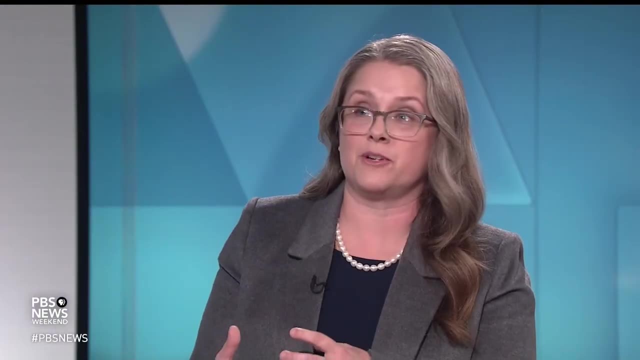 And then that campaign went around the country, around the globe, And generations later, medical school students are more likely to learn about polio in history books than they are in clinic here in the US, And that's because of that work. It didn't just go away because we 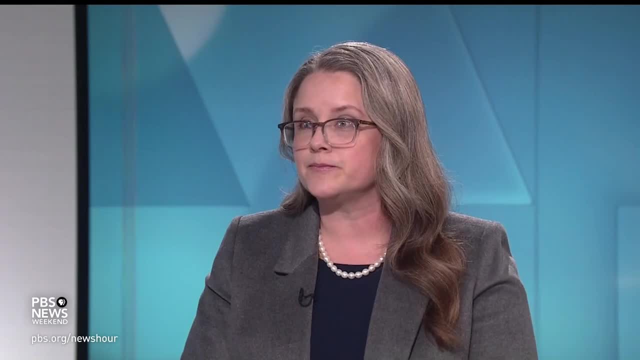 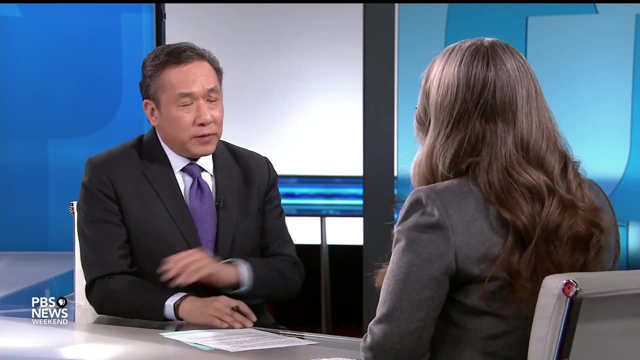 wished it away. It went away because of these vaccine campaigns. JOHN YANG, And how did all the disinformation that spread and the mistrust that spread around the COVID vaccine? how has that affected other vaccines? LAURA BARRON- You know we have been dealing with misinformation for quite some time. when it comes 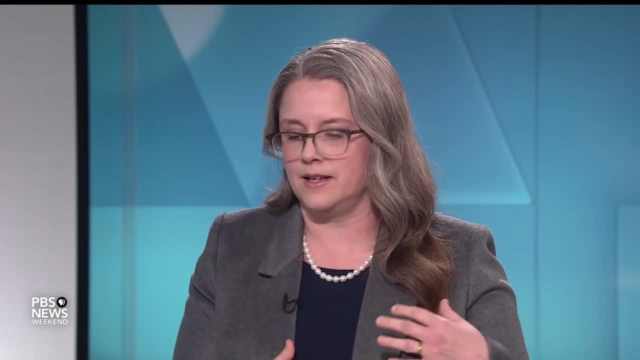 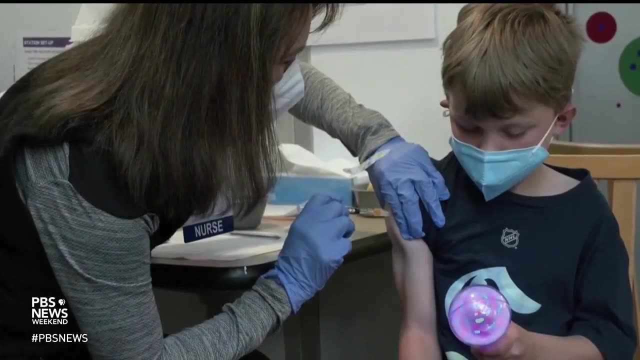 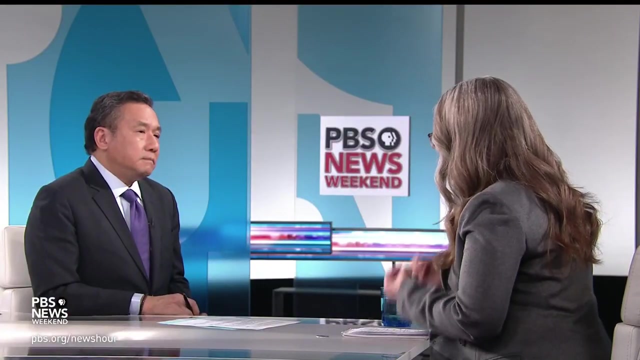 to vaccines. you know, starting in the late 1990s thinking about the measles, mumps, rubella vaccine, And to this day there are still people who withhold that vaccine from their children because they think it might cause problems. that just evidence studies conducted over so many years. 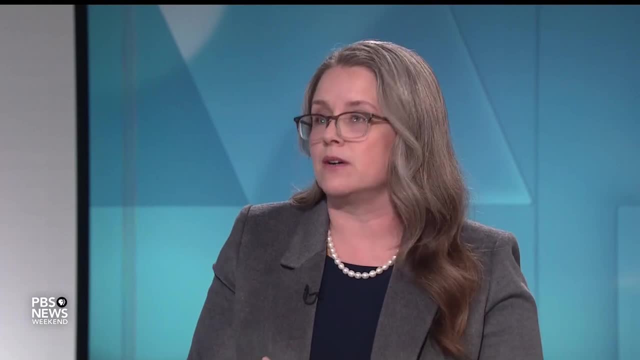 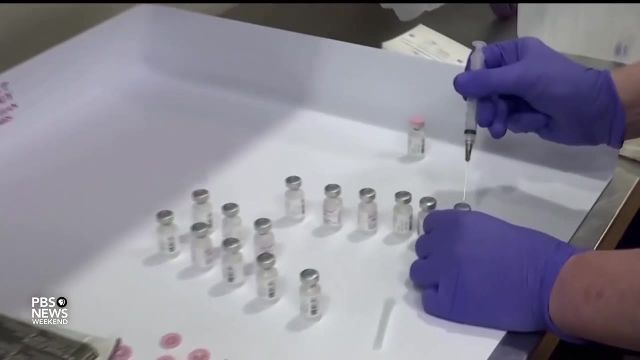 in so many countries. just they continue to debunk that since-retracted study. But that sort of laid the groundwork for some of the misinformation campaigns we're seeing about COVID vaccine now, whether it's talking about how quickly it was deployed, And then when politics are getting involved in some of those campaigns. 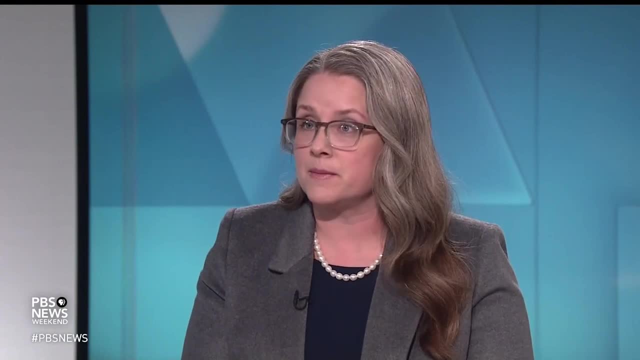 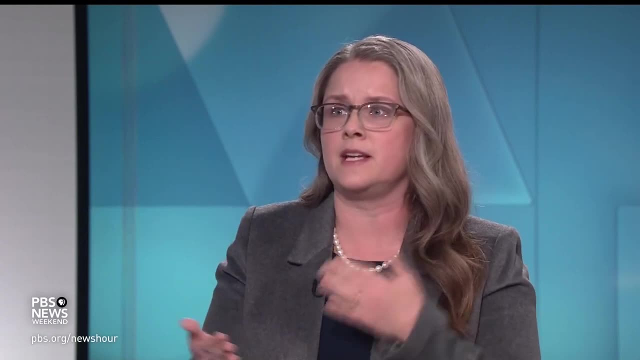 it makes it a mess to disentangle. Time and again when I have been talking to clinicians about this, they recommend that people ask their doctors if you have questions about the COVID vaccine, measles vaccine, any of these vaccines that are recommended, that are approved and vetted. 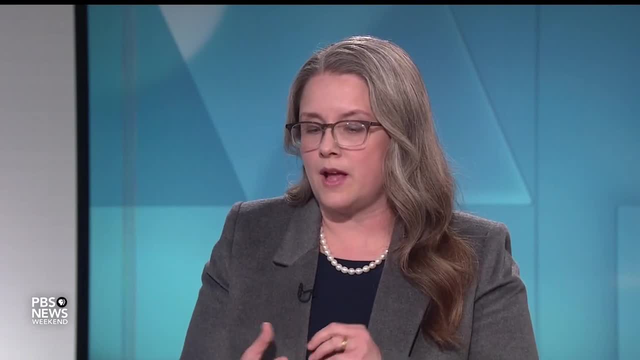 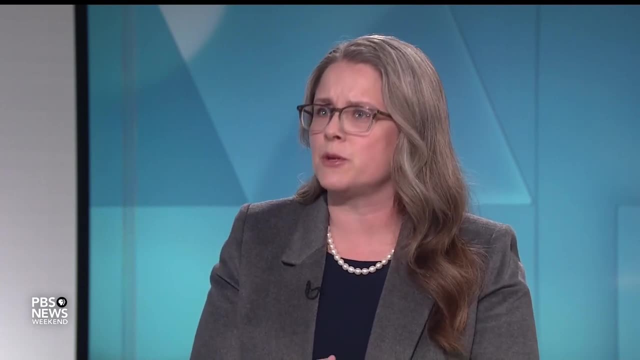 by the CDC, by the FDA. have those conversations with your doctors. but also, perhaps equally important, LISA DESJARDINS, Certainly Doctors should be ready to have those conversations with their patients. I had a conversation with a doctor in South Alabama who was saying: 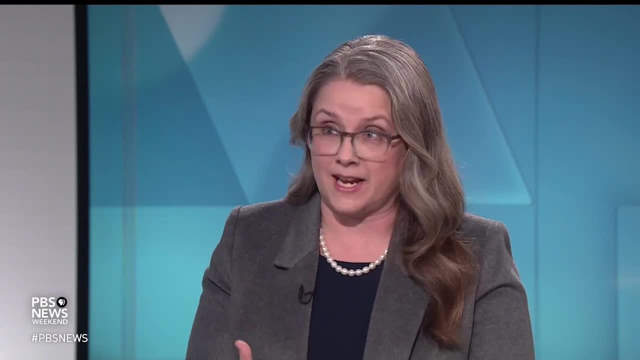 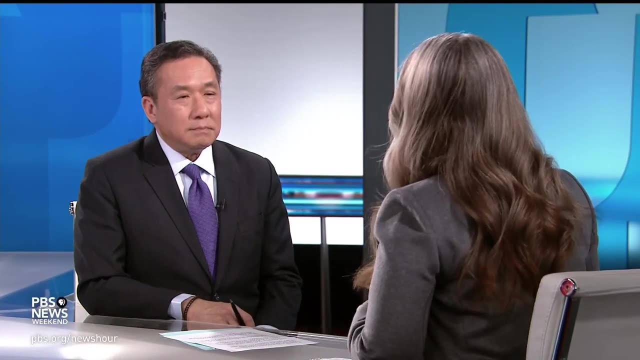 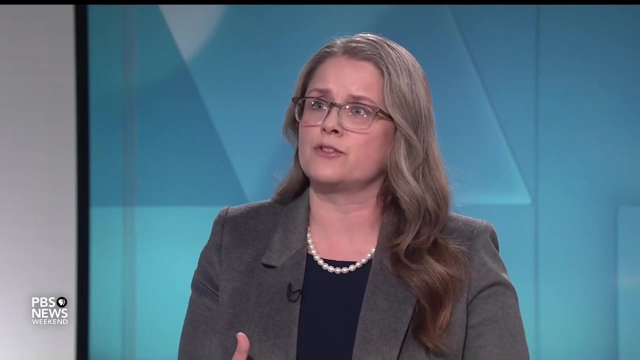 physicians should be welcoming these conversations. They should be ready to answer questions and shouldn't discourage patients from having them in the first place. Vaccine misinformation expert also told me that people are going to misinformation for a number of reasons, but some of those reasons is because they weren't able to get answers when they 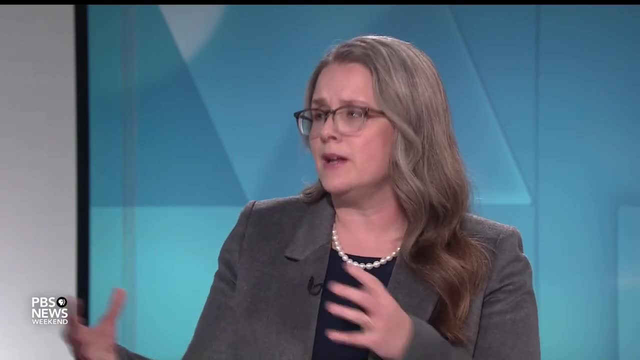 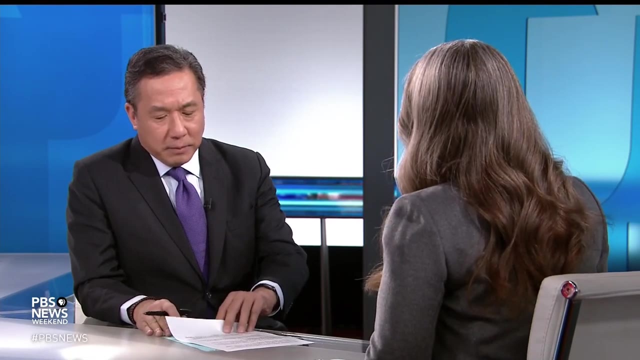 needed them from their health care providers in the first place. So just be ready to have these conversations and welcome them. JOHN YANG, What are the fears that you have heard from doctors and public health officials about this, about diseases that we thought we had conquered? 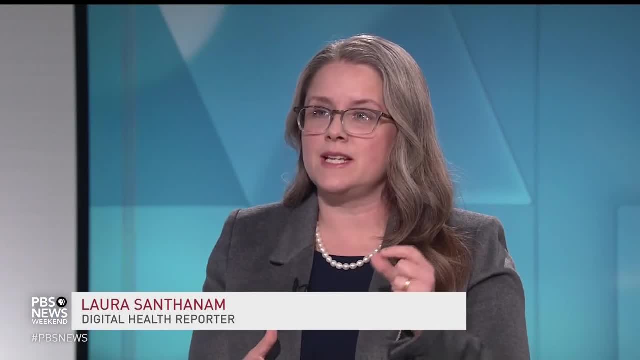 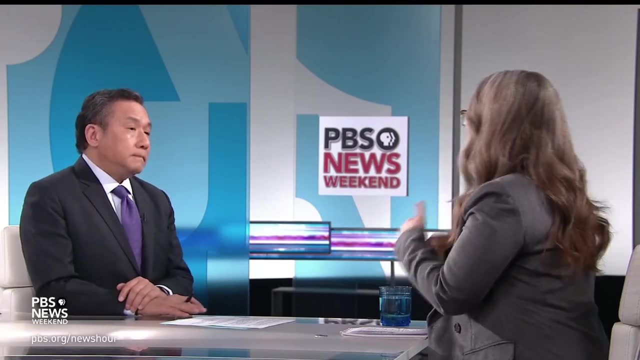 that have been wiped out, like measles, LISA, DESJARDINS. In the US we have seen vaccination rates among kindergarteners decline to 93 percent. It's supposed to be 95 percent, right, That's the recommended. 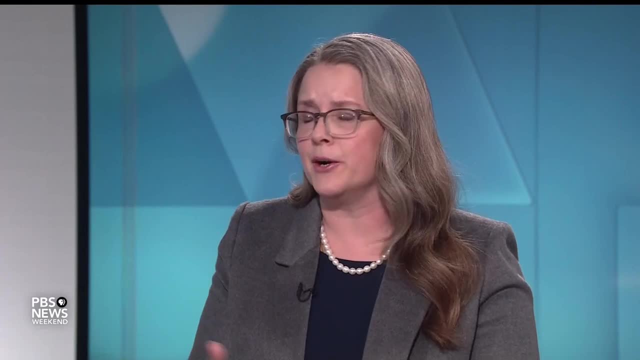 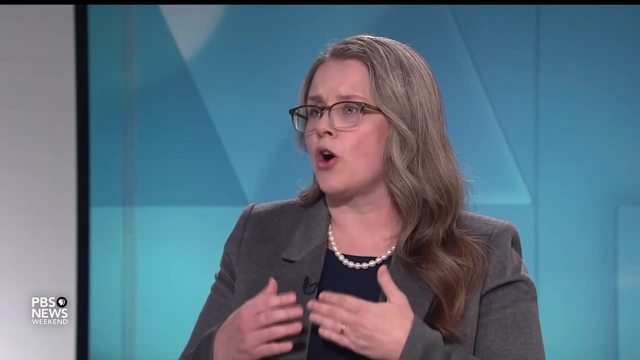 threshold to prevent community transmission and a lot of suffering and harm. Two percentage points may not sound like a lot, but according to the CDC that roughly translates to 150,000 kids who are left at higher risk for developing measles. They could become deaf as a result, develop encephalitis and, in most tragic cases, die. Physicians, pediatricians especially, who I have talked to in my reporting, are very concerned that we will give a foothold to these diseases that we had worked so hard. 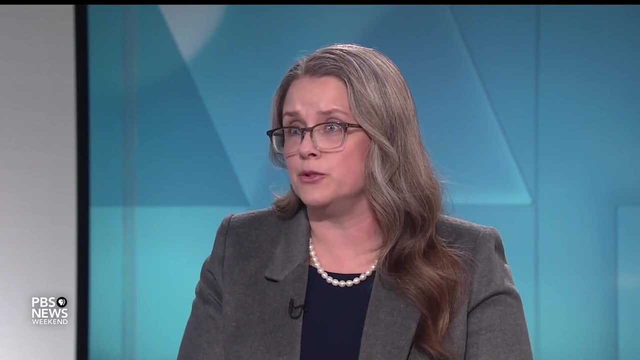 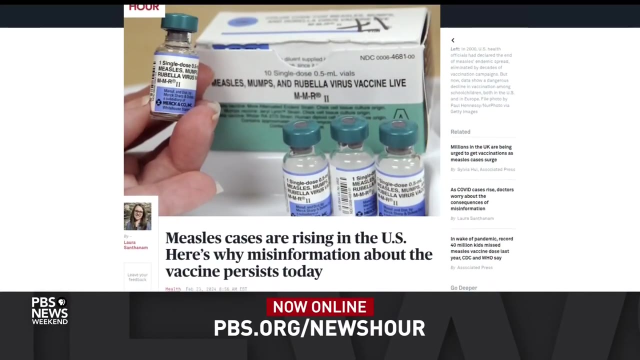 to contain that will give an opportunity for preventable death to rise in this country. JOHN YANG, Laura Santana, our digital health reporter. thank you very much, LISA DESJARDINS. Thank you, JOHN YANG. And you can read more of Laura's reporting on the rise in measles cases and: